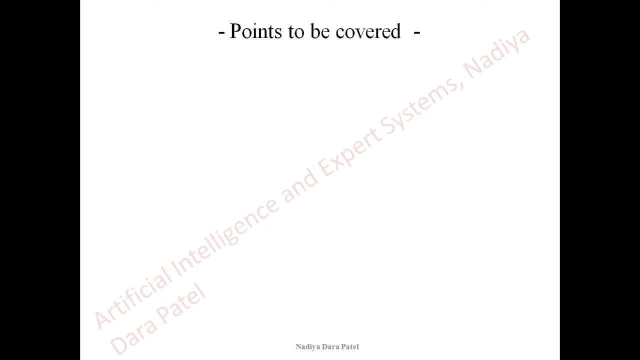 intelligence and embedded into machines. So points we are going to cover in today's lecture are going to be the next component of intelligence, which is perception. We have already seen two, three components of intelligence and now in today's lecture we will speak about perception. It's short introduction Before directly studying the concept and technical. 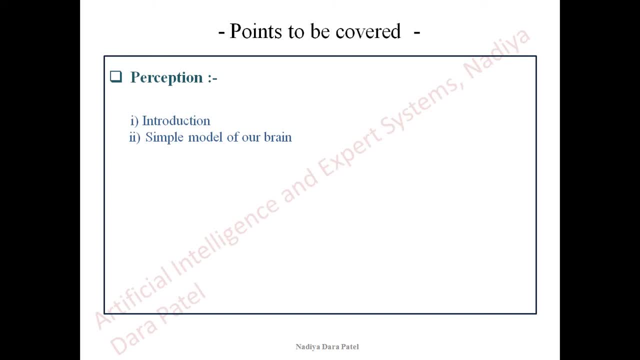 terms of intelligence, we are going to talk about the concept of perception. We are going to talk about the concept of intelligence and we are going to talk about the concept of perception. So, in terms and the working of perception, we will see a small simulation, or: 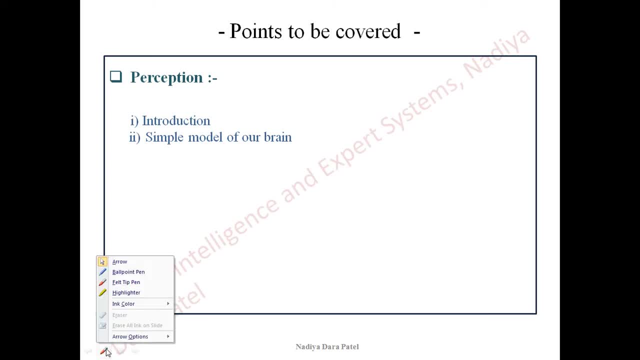 simple model of our brain so that we can understand how exactly human perception works. and once we understand what human perception is all about, we will then map or study the perception in terms of technicalities and in terms of artificial intelligence algorithms. Further we will see definition of perception and 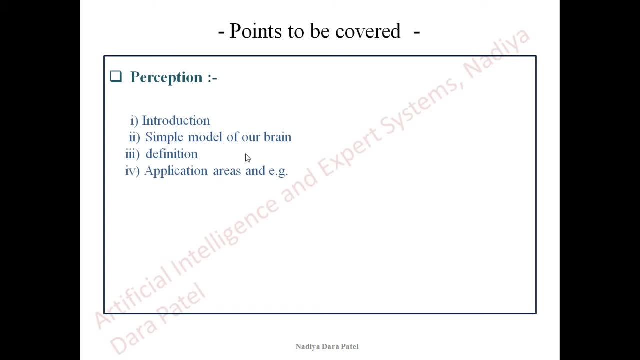 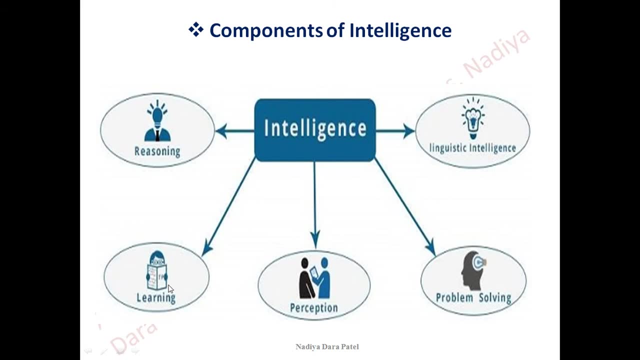 finally, application areas and one or two examples of perception. So we have already seen what reasoning is, what learning is, what problem solving in artificial intelligence or component of intelligence is, and now, finally, we will study what perception is. So, before starting, I would like to tell you that perception is that very component of intelligence and it is a very 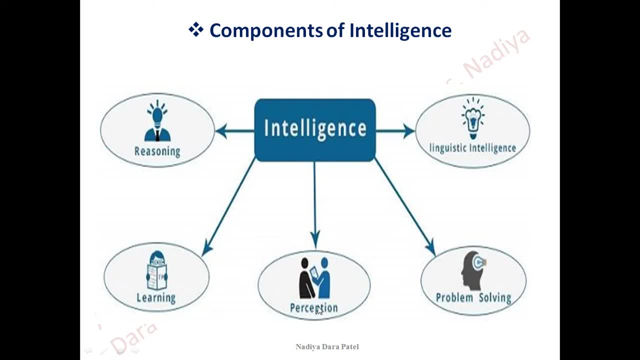 basic component which has actually taken machines very close to humans and human intelligence. So this is a- you can say basic part of our intelligence which is by far we can say the daily course, or you can say the something which is a part and parcel of our daily routine. So you don't need to have 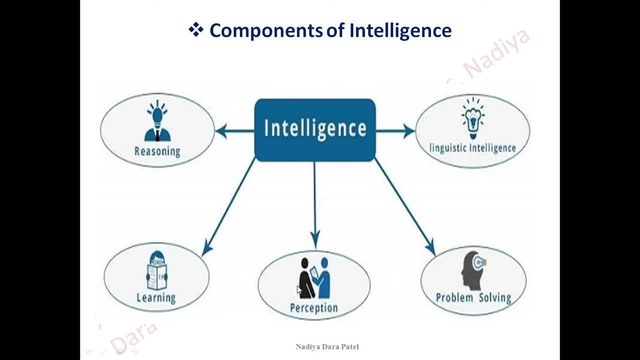 an expertise over some part of brain. If somebody is expert, his brain is expert. his brain is expert, his perception is good. It is something which is a part of our daily life. So these are the basic functioning and this is the primary, you can say, component of intelligence which got transformed. 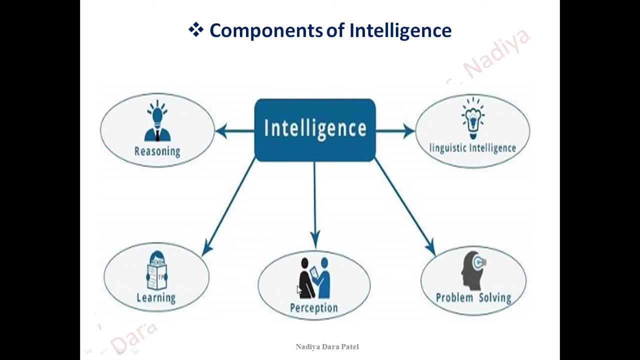 in artificial intelligence very early. So the first thing which they started building on was perception, and then it was very successful but it had some very limited kind of functionality. But it was a huge achievement in the field of artificial intelligence back into the previous years and further then with the course of advancement, they came up with new technologies. 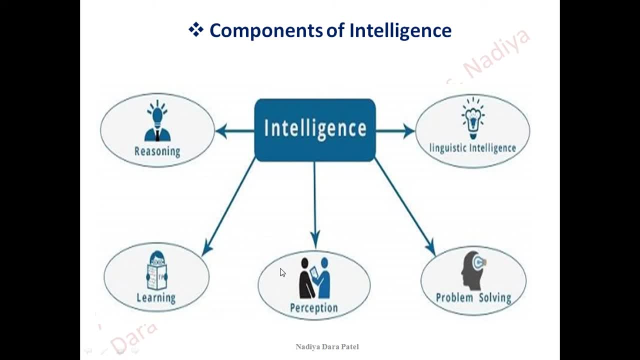 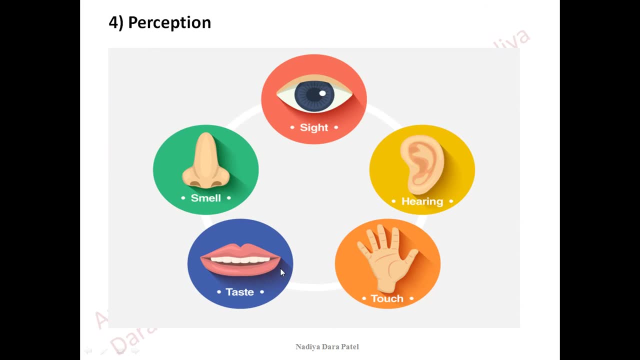 and new parts which could build this very component of intelligence and take machines closer to humans. So, speaking into basic terms, or you can say biological terms, what is perception? So, as you can see, we can say that perception is a part of our daily life. So what is perception? So, as you, 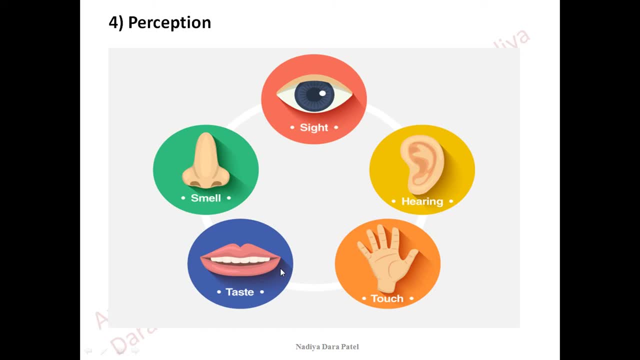 can see, we can say that perception is a part of our daily life. So, as you can see, we can say that you can see five senses in front of you on the screen. So there is sight, there is hearing, there is smell, taste and finally, touch. So these are the five senses which we all have. 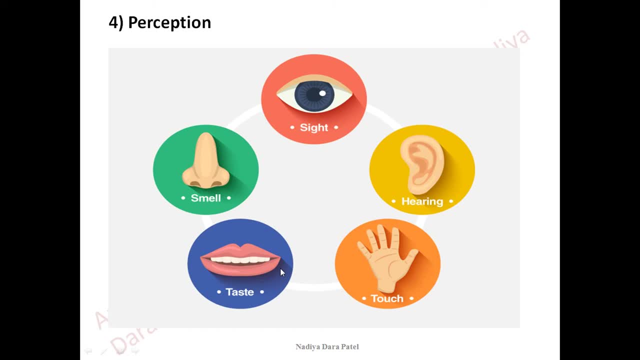 We are blessed that we all have got all of these senses. There are some people who are deprived of these basic senses too, but still they manage to live a normal life. So we can say that normal life just like us, by making the other senses strong. Say, for example, there is a person 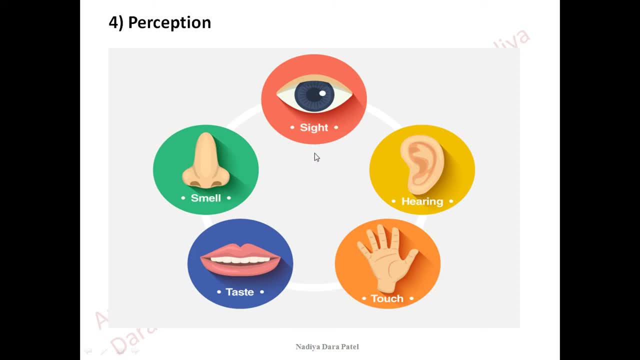 who is not having right amount of vision or is having a problem in his eyesight. At such situations, that very person is trained to make the rest of the senses stronger. So a person who is not having vision will definitely have a beautiful capacity of hearing- a way better. 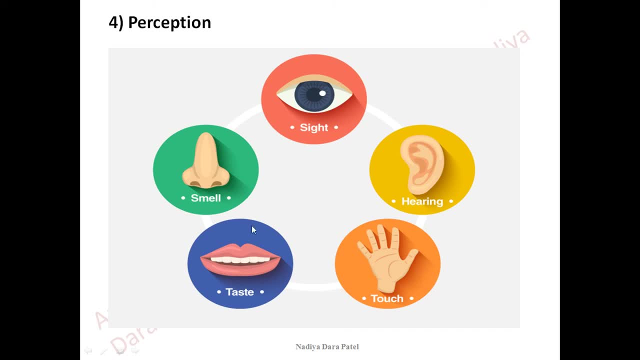 capacity of touch and will definitely have taste and smell far more better than us, which are normal people. So whenever you see some people who are not having the basic or one of the sense, they will definitely have the rest of the senses, which will be far more better or best designed. 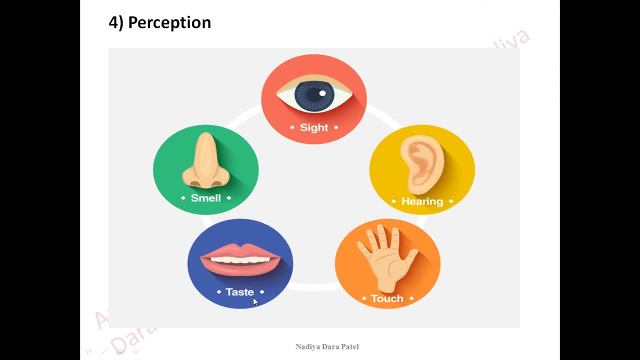 than you. So these are the five components which help build perception. So if you have sight, we see. we capture the objects. we capture them in the form of patterns, we recall the pattern. So it is not just like you are just watching and just forgetting, not like that With the time. 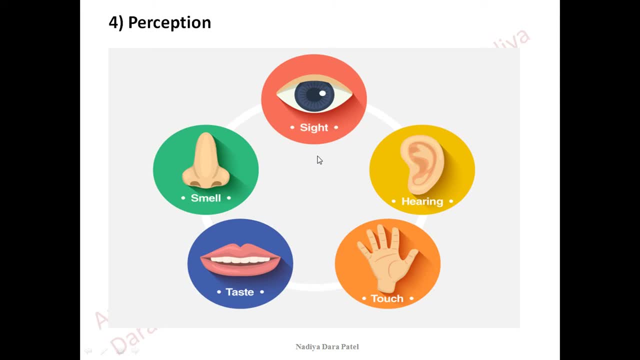 we apply this pattern to recognize the similar objects. So this is vision. Hearing is another capability. When it comes to hearing, you can say it to only listening. but not only listening, you can have or you can actually recognize voices. So say, for example, your friend calls you up. 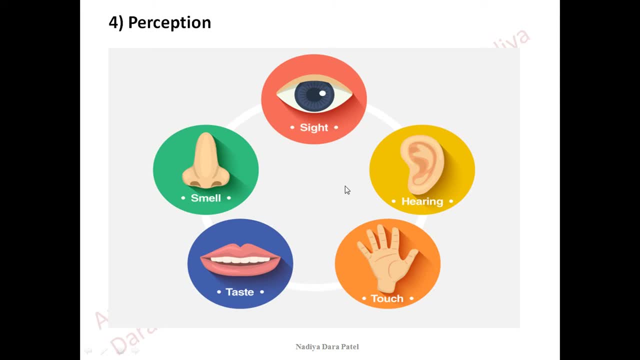 with some another number and fakes to be somebody different, but you can still recognize his or her voice that this is my best friend calling from some another number and trying to make a fool out of me. So this is the hearing capability. You can actually recognize the same voice, but you can. 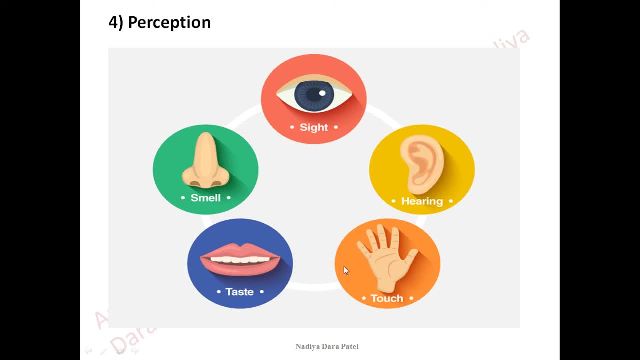 feel, you can touch things and actually recognize that. Say, for example, fabric, If you close your eyes and just feel a fabric and try to analyze whether what type of fabric it is. So this is one example With the same thing: taste- If you get blindfolded and you taste something you can. 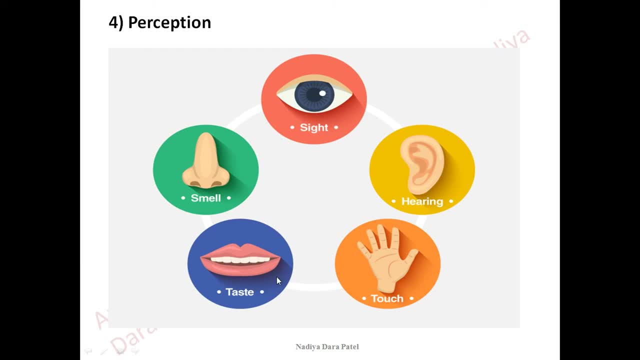 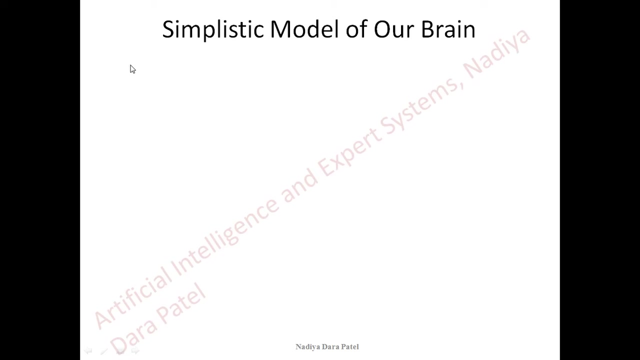 definitely recall that this is something which my mom has prepared for me. So the taste, So these are the senses which work together or separately And form perception. So, speaking in more biological terms, and if we apply the same in the term of brain, I'll give you certain examples. Say, for example, I can remember a song's tune more, better. 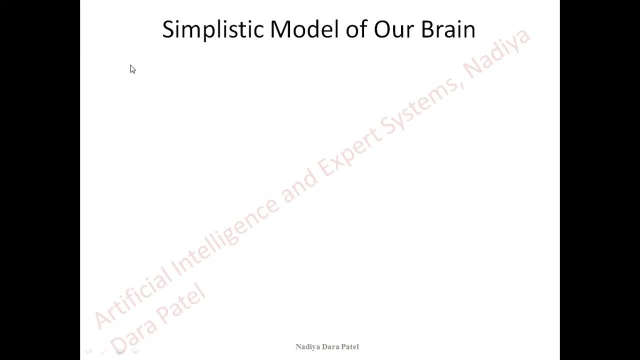 than the lyrics. Maybe I forget the lyrics. I just maybe recognize or memorize only one or two lines of a song, but I definitely Know the composed tune till the end. I know the music behind it. Similarly, I can recognize faces. 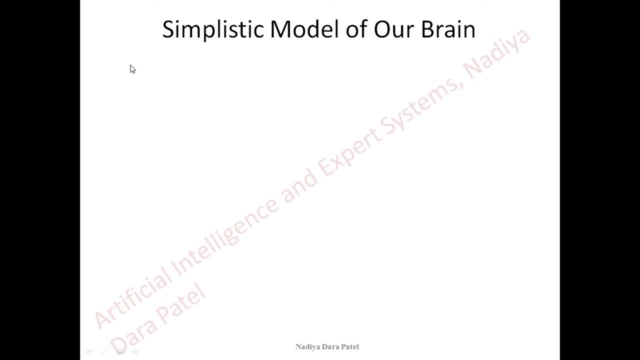 more better than the names. I maybe I'm not good at remembering somebody's name, but I can definitely recognize his face. If the same person meets me after 10 or 15 years, I'll recognize that person but will not recognize his name, Probably Similarly. one more example which I gave you: 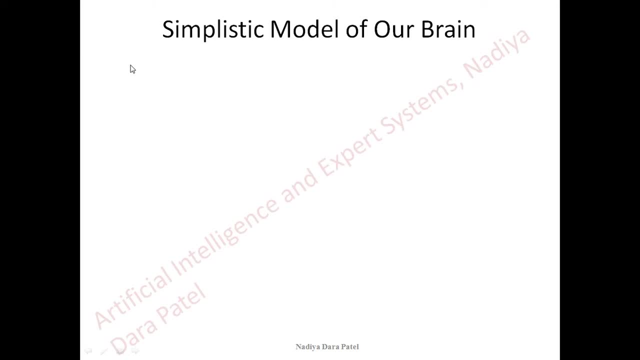 If I close my Eyes and try to feel a fabric, I can actually make out whether the fabric is silk or it is cotton. I don't have to see it, I don't have to watch it actually, but I can feel it with my hands. 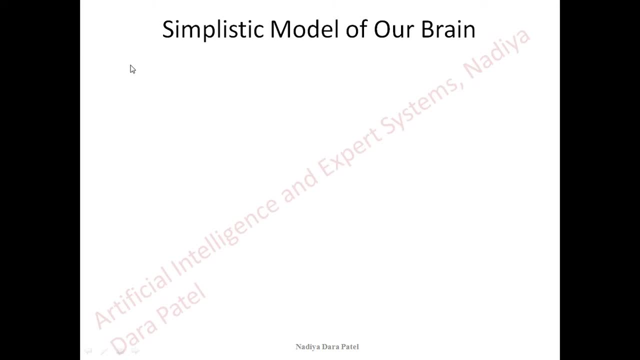 So taking into conclusions, then if I'm not able to recognize somebody's name, that means maybe I am less intelligent. If I am Not able to Recognize or remember lyrics of a song, of a song, does that mean that I am a bad learner? then? 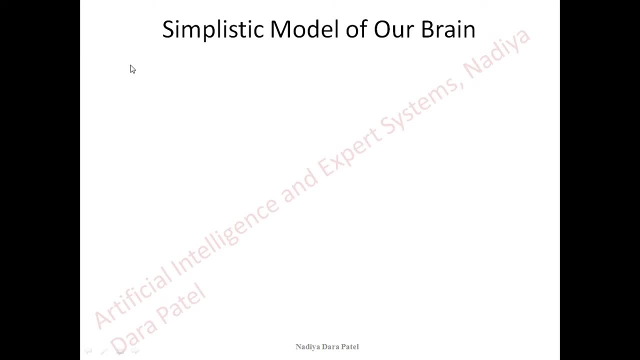 At the same time. maybe sometimes I can taste some food but not exactly tell you the recipe or not exactly tell you what is inside it, Like there are some people who can taste something into a restaurant and quickly will head in their kitchen and prepare the same dish as it is. 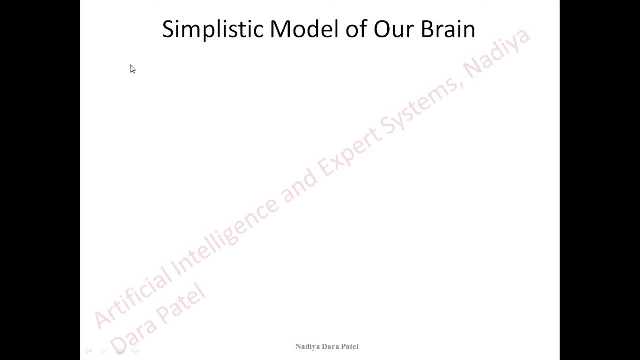 So These people are very good at taste, so they know what components makes, or you can say tastes once it is cooked or once it is uncooked. So maybe I'm not good at it, but I can recognize what the taste it is having. 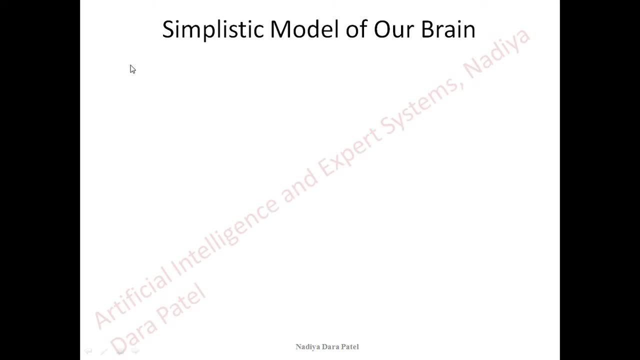 I can find the major ingredients which it is having, but not particularly. I cannot write down a recipe for you for a particular dish. So it's the thing that maybe I am not a good learner. Similarly, while studies, i recall and remember diagrams as it is, so i don't have to stress or i don't need 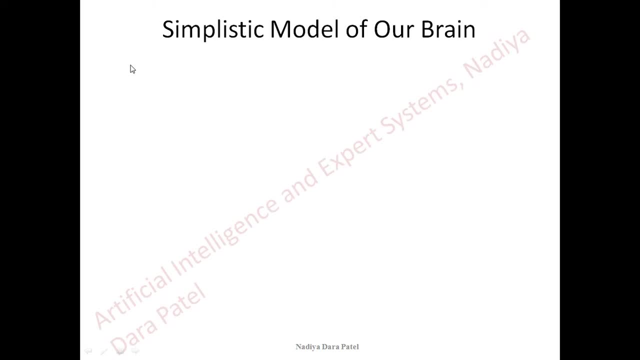 that extra attention or extra practice to perform or study and memorize diagrams. i can see it for once, i can practice it for a couple of times and that's it. i can remember it for life. so i'm good at diagrams? maybe, but if you ask me to write down a piece, a theory from my textbook or from my 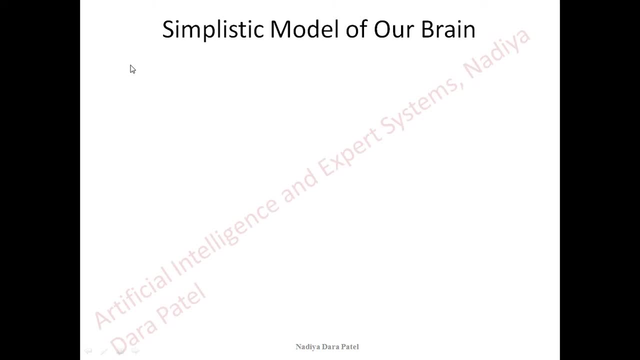 reference book, some definitions with the same words, same sentences, same framing of the paragraphs. i may fail. i am not that kind of a person which is good at memorizing things into paragraphs and write it down again after some days or years, but rather i can understand and write them in my own. 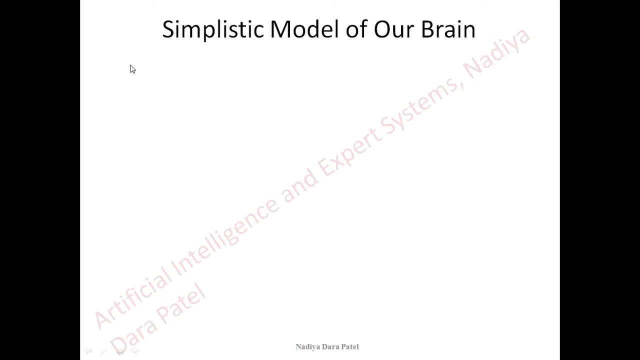 words, so i can do that. but one thing which i have noted about me is i can recall diagrams very quickly and remember. if you have given me some patterns and diagram and labels, i'll remember it as it is. so is this thing concluding that i am not a good learner? actually, the thing is, our brain is divided. 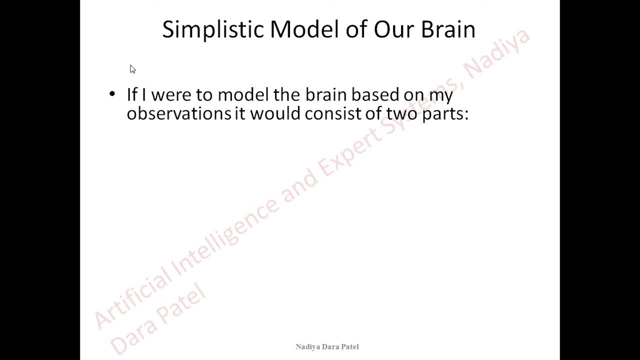 basically, but it has got many dividations. but basically we can divide it into two parts. the first part is the right side, which is good at perception, and the second part is the left side, which is majorly known as rational part. so this perception part is actually based on the things i told you. 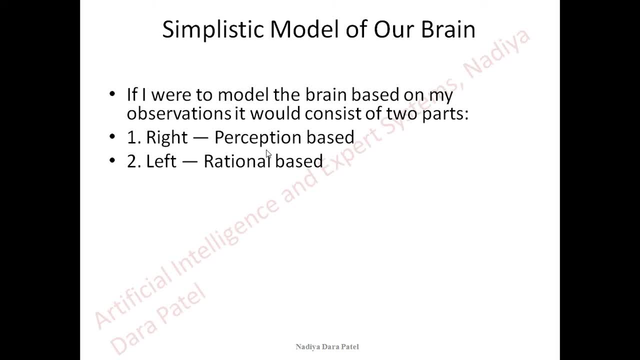 like i can recall diagram beautifully. i can recall a song's tune but not the lyrics. so the rational part is something where your logical things reside. as i told you that i can recall a diagram, but when it comes to recalling a formula, a mathematical formula or integration, and 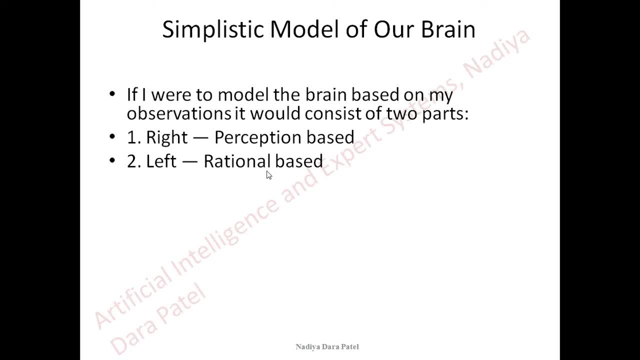 derivation formulas. i fail. when it comes to recalling chemistry reactions and equations, i fail. so this is that part of brain where logical things come up and these logical things reside in the logical logical things left side of your brain. so whatever textual material, like i told you the definitions which 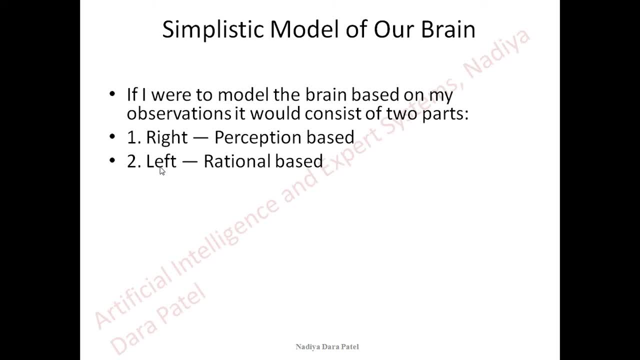 we study in our reference books, the paragraphs which we study and we write down in our exams. all this textual framing or textual things reside in the left side of the brain and on the right side resides the- you can say the diagram, diagrams the artistic nature or artistic view. 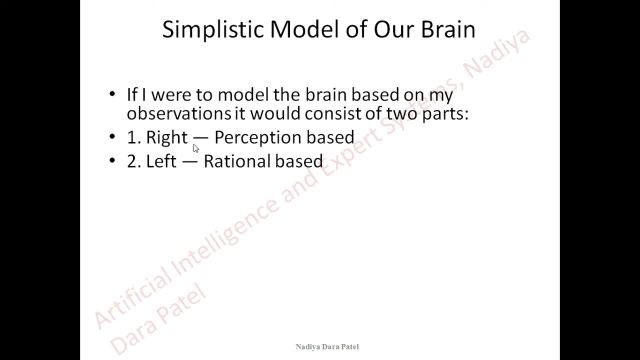 the people are good at singing, dancing, painting, actually are assumed to have their right side of brain to be a little bit active than the left side. so this is what happens, and this is the reason why we sometimes recall the tune of the song but not the lyrics. 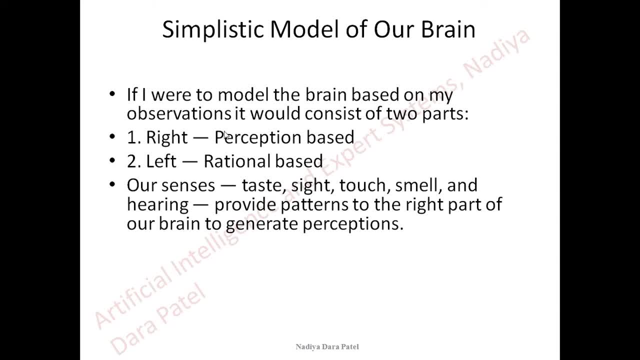 lyrics. because these two things are stored in the different parts of the brain. maybe the tune gets stored in the right and the lyrics gets stored in the left, and this tuning is very important when your left and right side of the brain functions very perfectly in synchronization you. 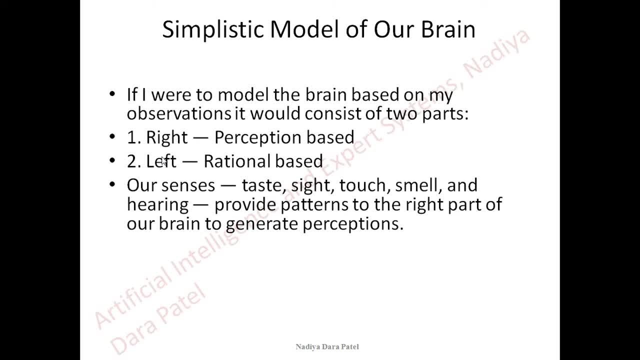 can sing with the tune and at the same time, even, i think, you can dance. you can sing in tune with all the notes, perfect the rhythm to be the perfect one, and also recall the dance steps which are in the song. so this is a very good part of the brain where both the sides of your brain 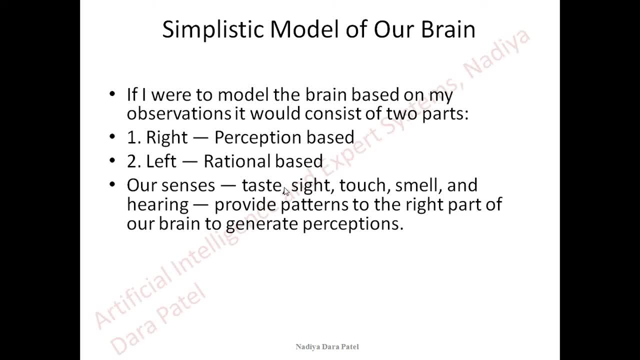 are functioning beautifully. so how does this actually happens? so, when you taste, sight or touch or smell and hear, these senses provides or creates first some patterns in the brain and which are stored in the right side, which is the perception side of the brain, to generate the perceptions. similarly, when it comes to logical interpretations, like i told you, if you ask me to, 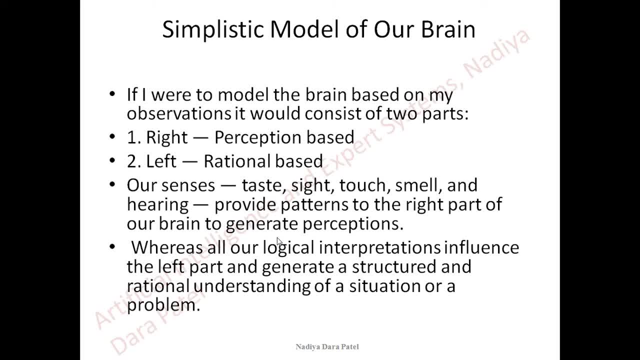 recall a formula from maths, i won't, but if you ask me to recall a diagram in maths which is little complex but still i'll remember it. so such logical interpretations are actually stored in the form of a structure which is the structure of the brain, which is the structure of the brain. 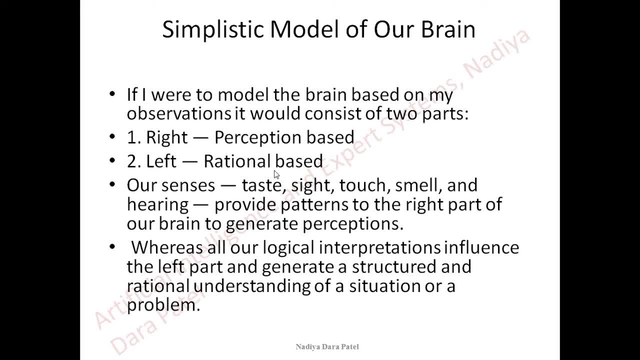 and rational understanding in the left side of the brain. so people who have both right and left in sync will be, you know, the so-called. i just actually don't like calling them intelligent, but okay, fine, these are the intelligent ones, and people like us, and me especially, who might have 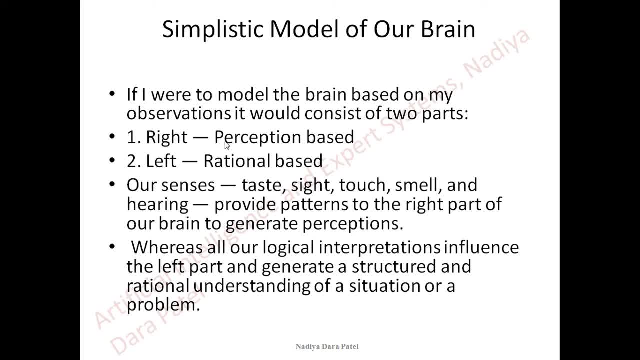 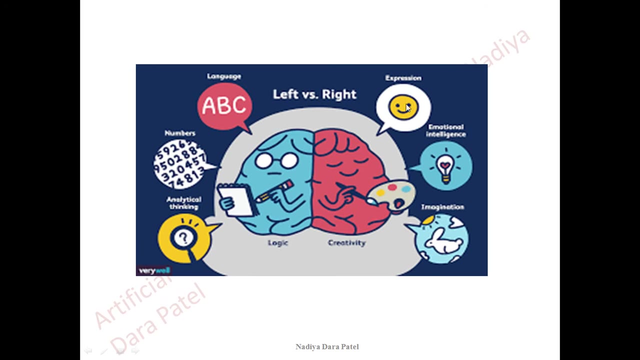 one side which is better than the other will have some parts or some components which we are good at. so that's it about human brain functioning. so this is what scientists and developers wanted to study and create in the form of component in machines. so this is how it works: the left side and the right. 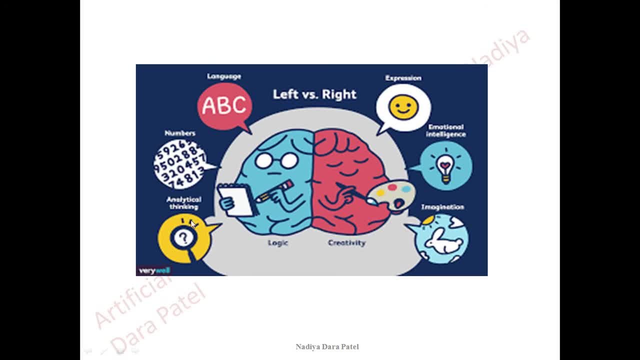 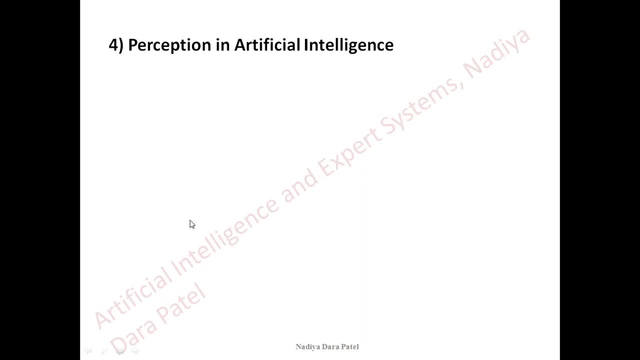 side, which contains the creative side, and this is the logical side. so what actually? now, perception in artificial intelligence is all about. so, speaking in terms of definition, machine perception or perception is the ability to use input from sensors. now, what are sensors, if you ask me? in humans, what are the sensors? 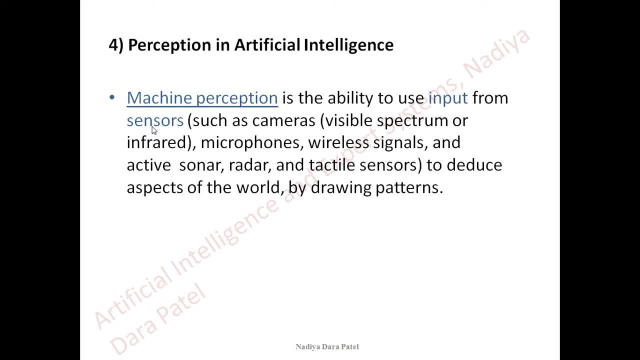 the organs which sense are sensors, but if you are supposed to transform it in the form of a machine, then you'll have to make use of some components or devices like cameras, camera visible spectrum or infrared, microphone, wireless signals, active sonar or radar, some tactile sensors which help in mobility, and these sensors actually sense, they provide input. 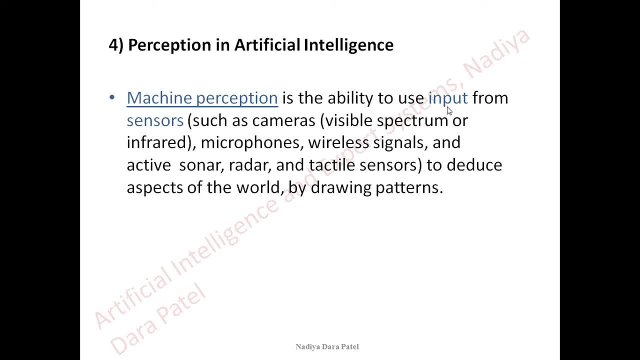 to a process or a program or an algorithm and it actually deduces. that means it reduces some aspects of the real world by drawing patterns. this is very important. by drawing patterns is it actually, you can say, saves its database for future. so one application which directly applies to perception is drawing patterns. 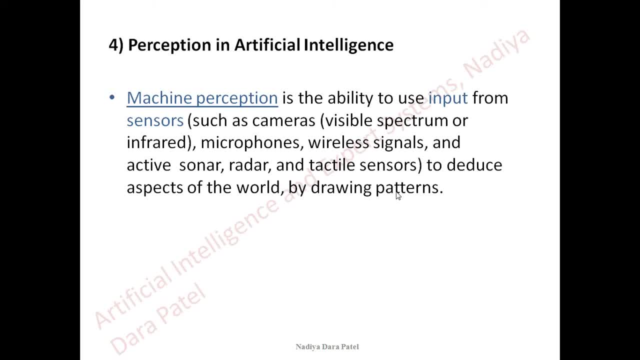 or you can say pattern recognition. it is a very important component of artificial intelligence when it comes to brain simulation. in perception, the elements actually scan any given environment by using different sense organs. these organs could be real or artificial, and the scene. so whenever a robot or a machine is supposed to sense, say for example, you're looking at this. 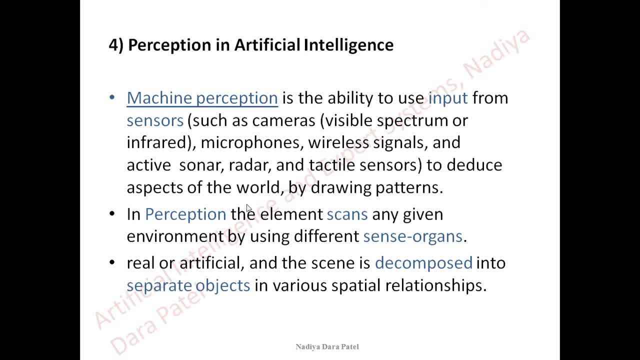 slide in front of you. so if you want to sense it, what you're supposed to do is draw patterns out of it and remember this whole screen. you're supposed to draw patterns out of it and remember this whole screen which is in front of you in the form of a scene. remember when we see some movies. say, for example: 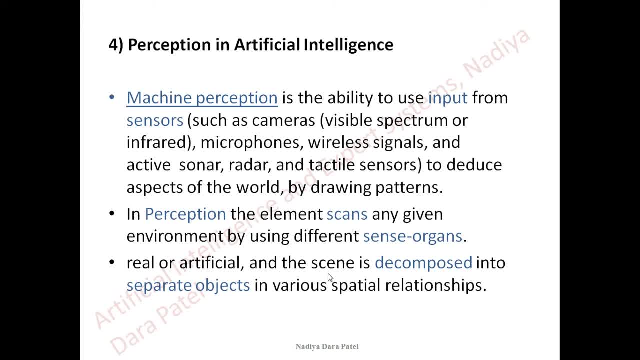 you have. you have your favorite movie on on your television. this is the second time you're watching it, but you will definitely know what scene is going to come next. so when objects move with sound and they have a voice, they have some music, they have some effects involved. 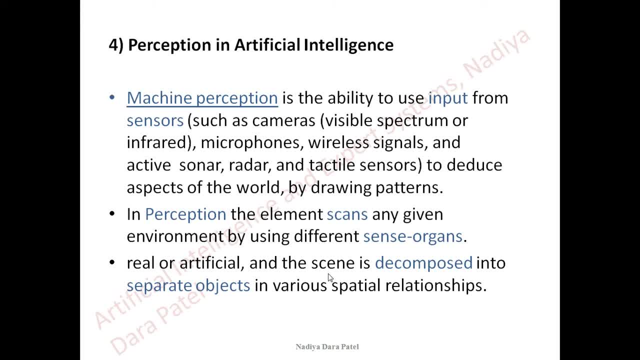 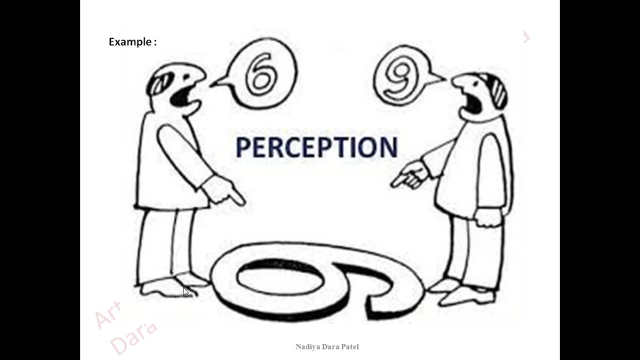 we recall them very perfectly, or you can say very easily: so machines actually senses objects and remembers them as a scene which is again decomposed into separate objects and into various spatial relationships. so one example here is perception. the another example, one we saw that we have our 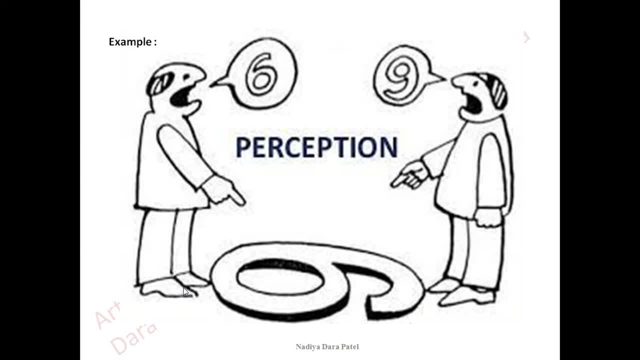 sensory organs which percept and gives impulses to the brain. the second example is this: the person is standing which is standing in the left side can actually see number six on the ground, but the person who is standing in the right side is actually having, or you can see, say that he is seeing- the number nine. this is a very popular 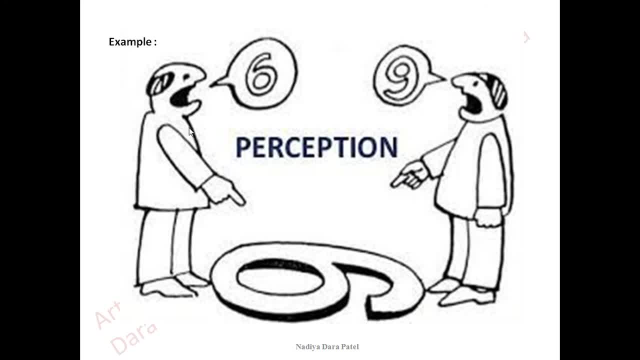 thing which went viral on social media, actually. so this is what perception means. so where you're standing, what you're watching, is not always the reality. if we ask both of them to interchange their positions, they will actually, you know, understand the other person was right and i was wrong. so many times when we percept, we actually assume and we actually start believing. 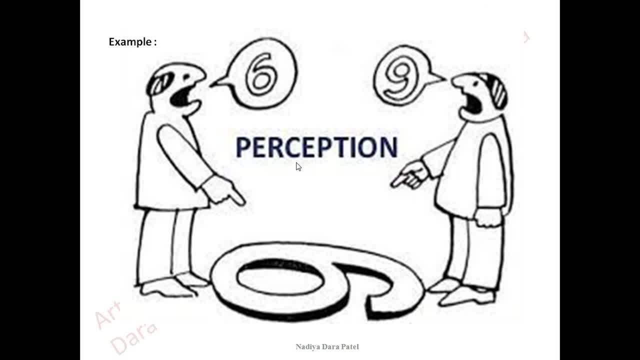 on something so many times, even in real life. we should try to change our perception. that is way of thinking towards life. so every time what you're assuming say: for example, there is a person in your classroom who is not friend with you, but still he is a part and you people are learning. 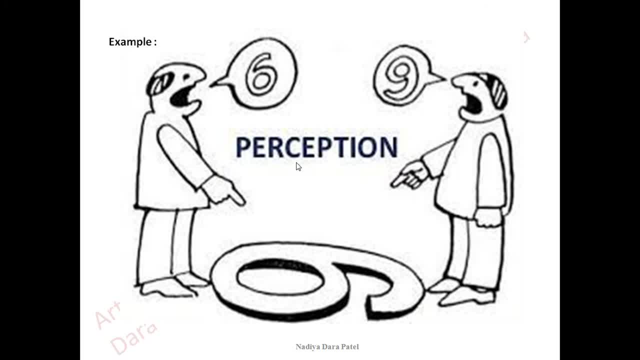 together from the last three years and is having a certain type of nature. you actually try to percept that maybe this is the thing and this is the problem, and this is the way this person is, but not really. that could not be reality. so change your way of thinking. 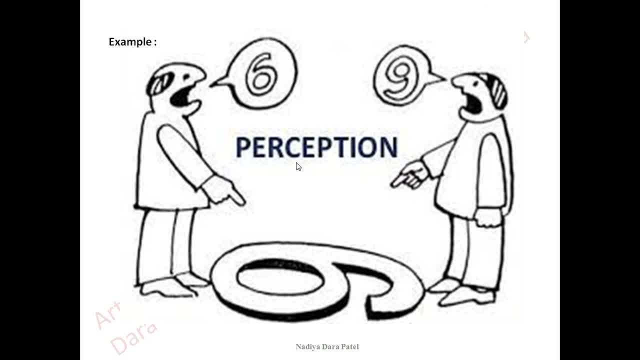 maybe the person is good, maybe the person can become your best friend in future. so this is what perception is. so many times, perception also depends on the positions, on the situations and on the objects. now this is one object which has got two perceptions. so if you see from this, 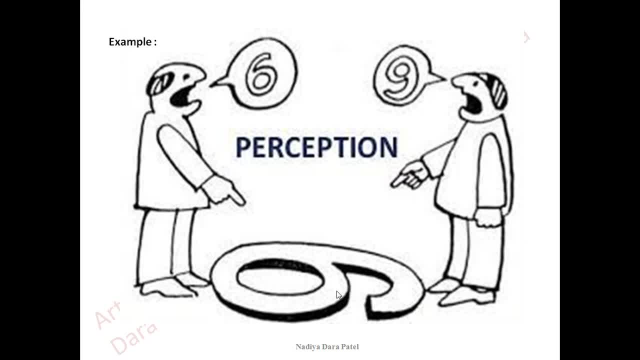 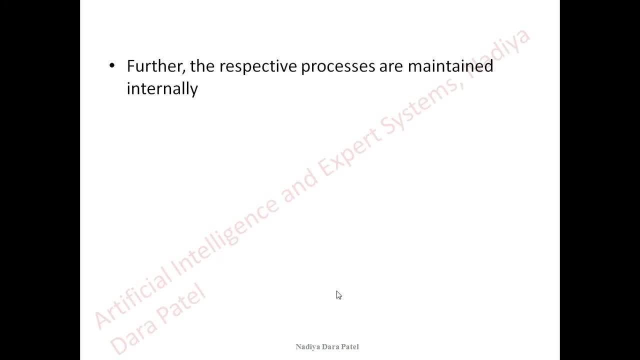 side, it is going to be different. if you see from this side, it is definitely going to be different. so, further, the respective processes, like the process which actually are saved, the process which contains the patterns, they are maintained internally, so these processes allow perceiver to analyze different scenes in the 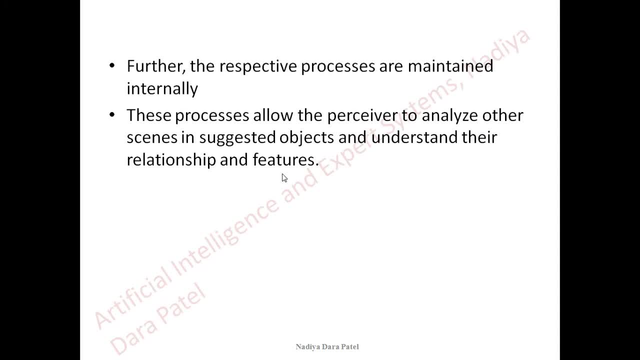 suggested object and understand their relationship and feature. like i told you, if we ask the people to interchange their positions, the perceiver will analyze other scene as well. this analysis is complicated as objects can be similar and can look different in different environment, like the number six and nine. this perception depends on the view, of the suggested angle and the perceiver. 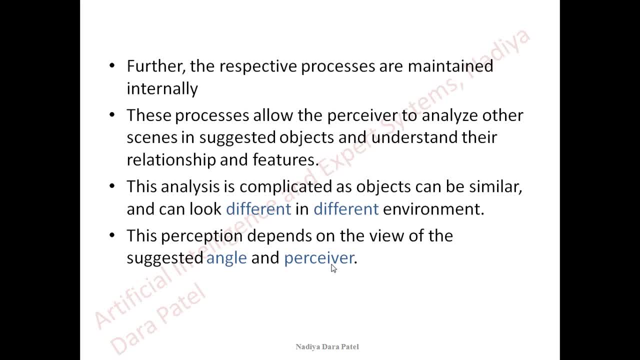 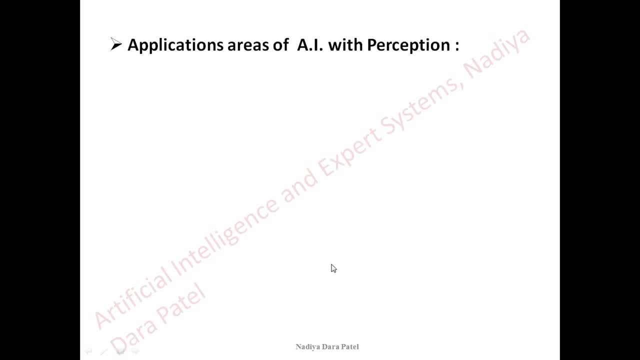 like the position left, you can see the number six and position right, you can see number nine. so what are application areas of artificial intelligence that are Lées, are kinda similar to that of durable robots like like aisttonides tripod that allows you to measure your motion. 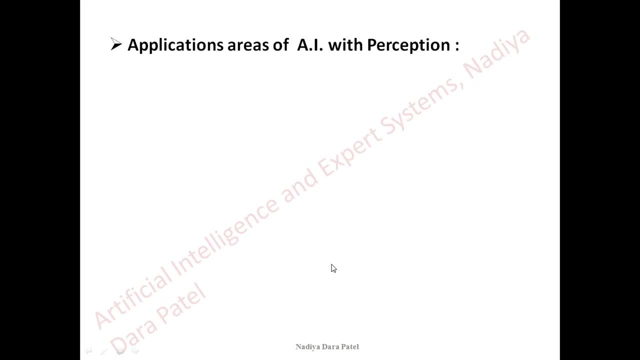 and you use your cognitive memory. we call it the throttle theory. the throttle theory that indicates a gaze and that in itself effectively examines the perception of a piece of object, something that looks at difference on the whole, and it require you to slowly look at the object based on the depth. 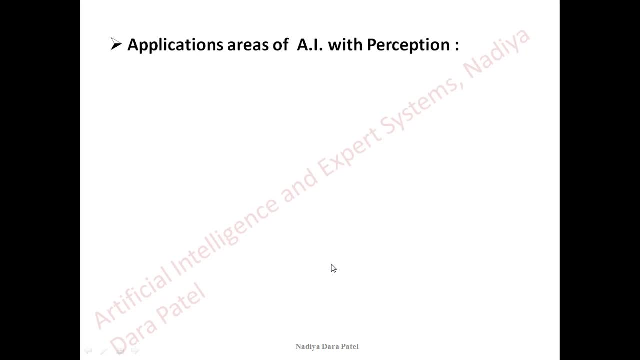 on theife, the conduct time of the object, you're not needed much of your attention in the practical aspect. then the platform field. the information about the object is marked. when you see this visual image, previbe your attention. there should be a figure in advance of the behaviour, that the behavior has to be recognized. 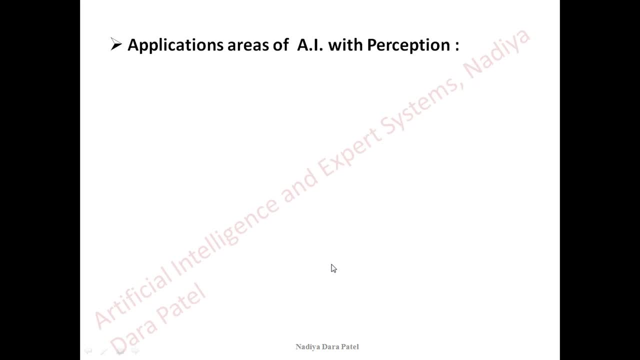 say that the object is a material and there is no decision about管 operating as a part of the engineering journey and the action. that is not something you have to do in such a relation like pattern. store them in your database and recall it timely, compare it every time you learn a new. 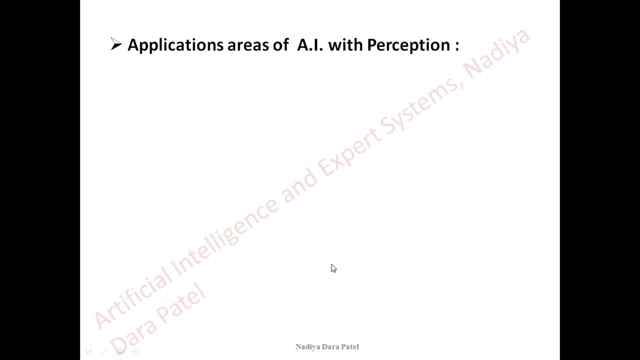 pattern. so pattern recognition is the field which directly applies to deep learning. so deep learning is where the devices actually mimic. if you have forgotten what deep learning and machine learning were, go back to our previous lecture and recall it, because that is going to help and that is the. 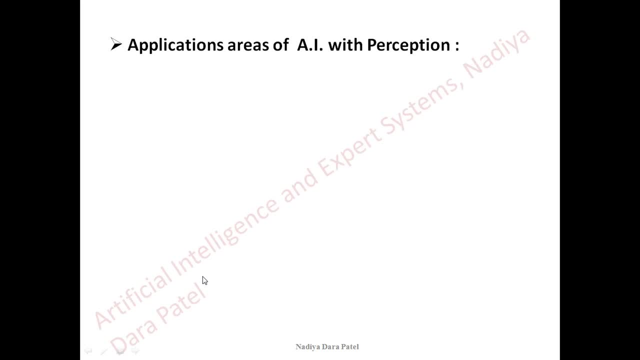 reason why i haven't added that part in this component, because you are supposed to write it down what deep learning is and what machine learning is and the. i forgot to keep a question mark here you are supposed to find the answer. perception will directly apply to deep learning. 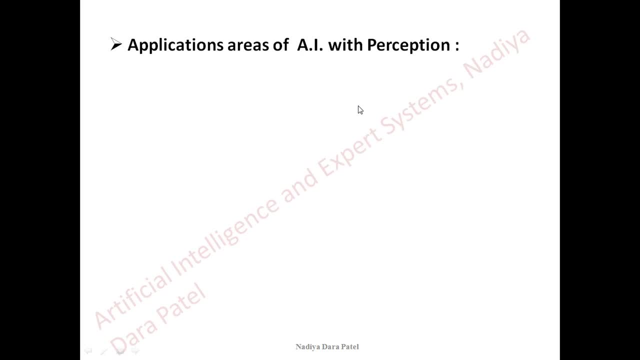 or perception will directly apply to machine learning. so one is deep learning, where you actually sit down, recognize pattern, store it in your database. next time when you standpoint an object, Say for example: first I just showed you a ball and in the second case I actually 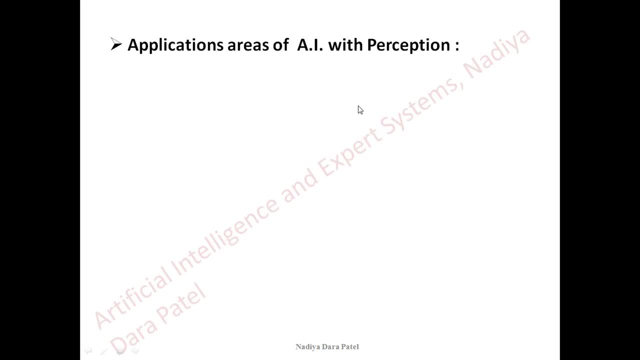 showed you the globe, the earth. Both the objects are having same shape when it comes to three dimension, but ball is different and globe is different. What makes it different is our perception. So this is what developers are expecting from robots. So some of the 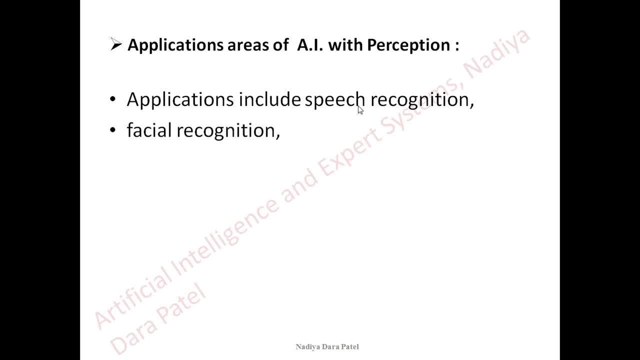 application area could be speech recognition, where you are supposed to recognize the speech and then translate it, or do the further operation. Facial recognition, as I told you, you are supposed to recognize an object, store its pattern in database and next time, when the same person comes up, you are supposed to match your database. 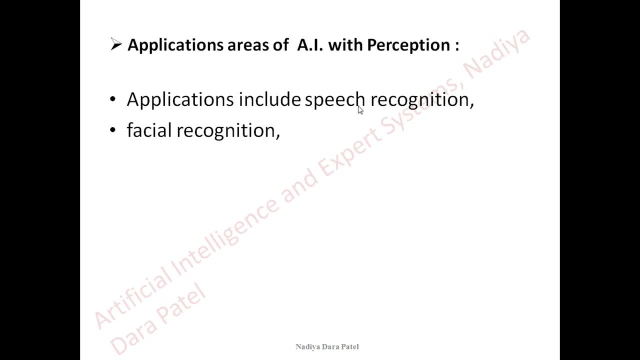 If it doesn't match your database, that means the person is new, which we already discussed about some lectures back where a person's passport had got rejected because face recognition software was not working properly. Imagine you have face recognition password in your mobile and it doesn't work, So that could be a very difficult situation for you to open. 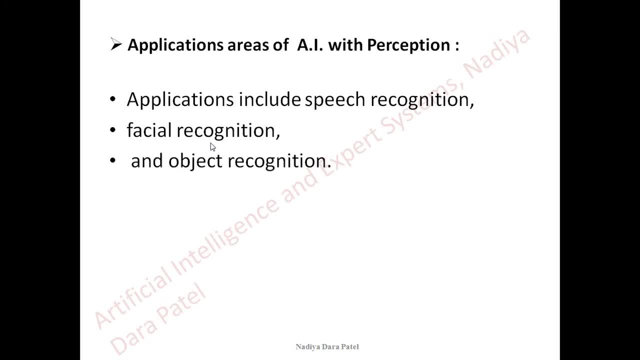 your phone. So this is where perception comes. object recognition, computer vision. so these are the application areas. So, looking about the example, as I told you that this was the very first component into design and it got designed very beautifully back some years back, many. 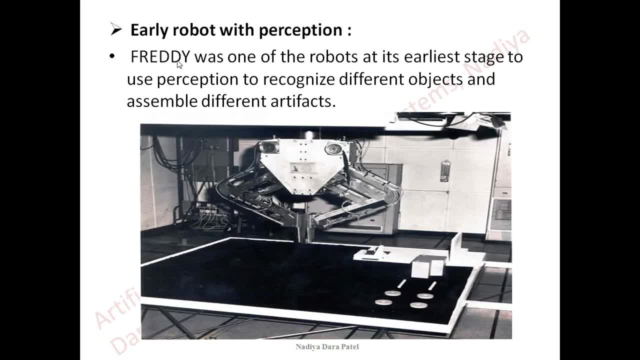 years back actually. So Freddy was one robot which got the perception. So this robot was actually not the typical robot. but this one was a factory robot with arms and locomotive skills and tactile things, given. it was supposed to recognize objects, like if i keep 10 objects in front of it, and i have programmed it. 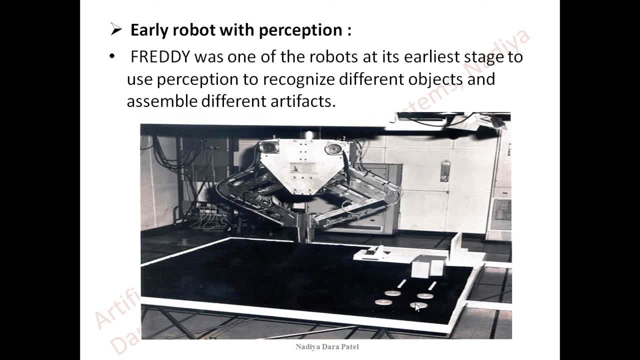 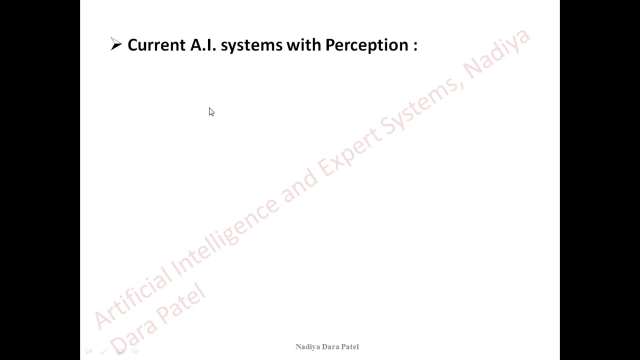 to pick up only toys from those objects. it will actually sense, through its sensors, recognize the object and pick it up. so this is what it used to do. so this was the early- you can say- advancement or the invention in perception. so current systems, if you ask me, which are good at perception is the 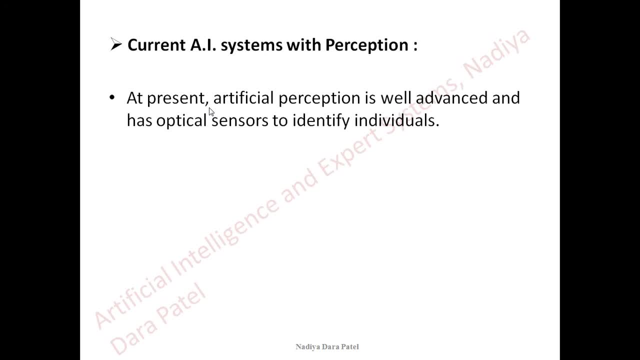 first one is which are good at optical sensors to identify individuals, like face recognition apps. the second very popular. the second very popular. the second very popular example is autonomous vehicles. the self-driving car have got or marked perception to the perfect stage so that they are driving into traffic oriented roads as well, in a moderate speed. but 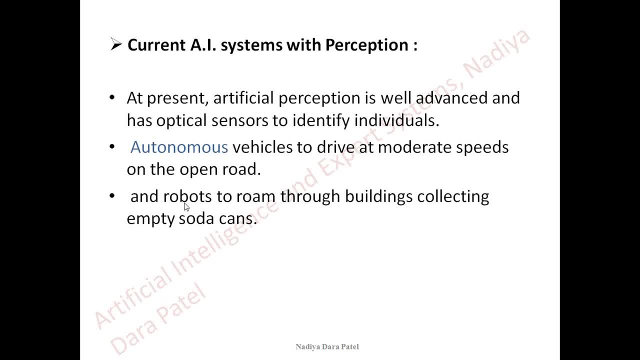 the next could be: yeah, this one again is a popular one, where the robots are actually trained to collect soda cans in foreign countries as well. i wish we have such a robots to clean our beaches, where plastic and other sewage things are actually blocking and making our aquatic animals die. so if we have got such robots which could clean the beaches by collecting 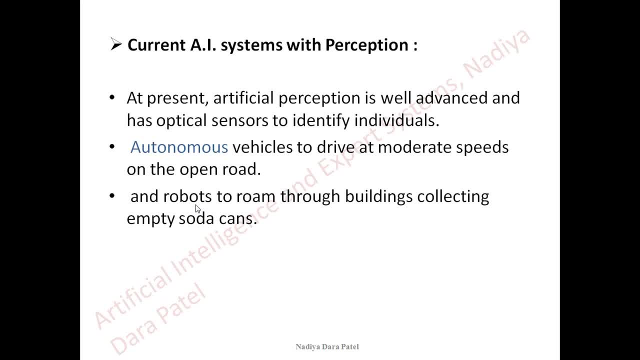 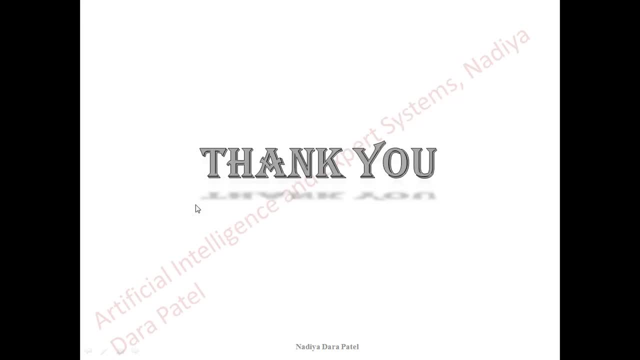 by sensing first and then collecting plastic. this could be like beautiful thing happening to us. so this is all about today's lecture perception. i hope it was easy and interesting. do not forget to go back and see whether deep learning would be the field or machine learning would be the field. thank you,